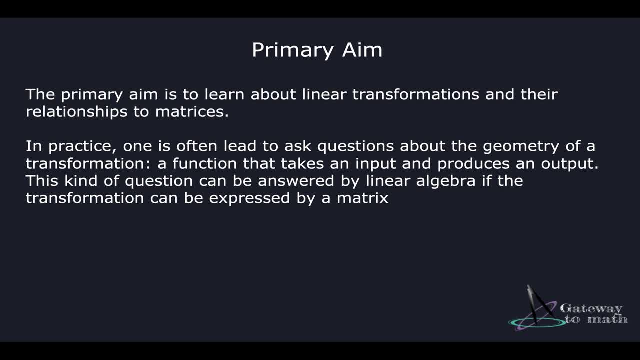 So it helps you make future predictions. I mean, let go of the math part of functions. Just think the day to day activity, all the actions that we ever do, all the beings doing any actions are a function. Why? Because you're plugging in some values and then you're getting the 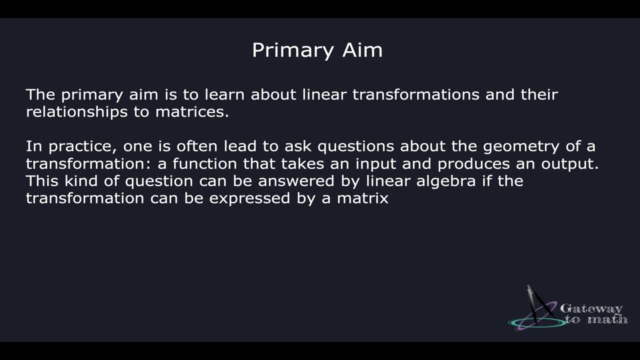 output. For instance, let us take an example of exercising. So if I'm exercising, my organs and body parts are moving and coordinating in some certain specific formats, right? So this becomes the input and then the output is a fit body, right? 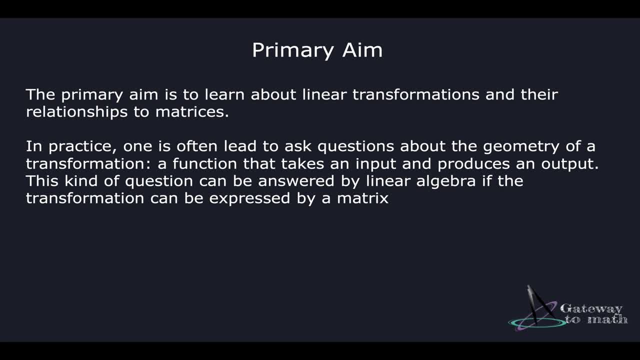 So any action that you do is a function, And since it is a function, that means whatever you give to it. that is, whatever actions you do, you will get the corresponding output, And that's how your life becomes, whatever day-to-day activities you do, right. 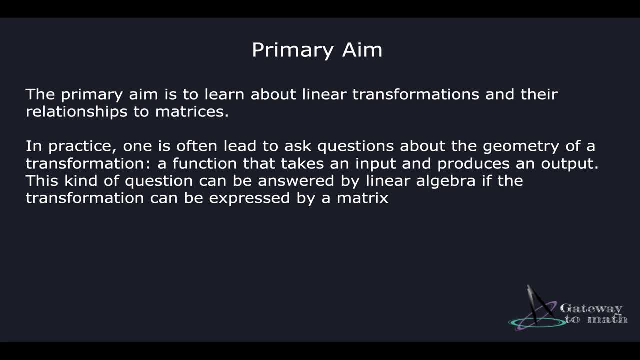 So you see how important the function is if you understand it mathematically and then apply it to day-to-day understanding. Okay, just an FYI: here I will be using two terms interchangeably: transformations and function, but they refer to one and the same thing. 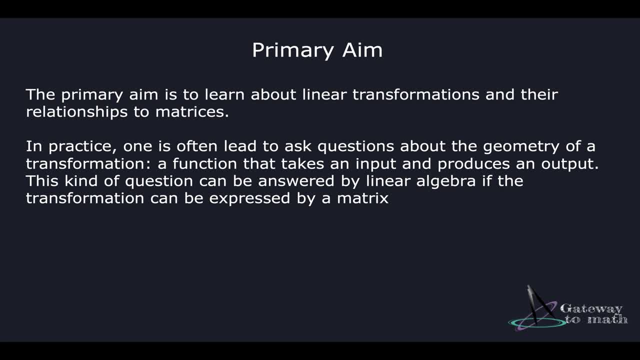 Transformation is just a little more fancy term to represent functions, but it's still the same thing, because you You take the input, you transform the input and then you get a different output. That is why the word transformation. So the primary aim is to learn about linear transformations and their relationships to matrices. 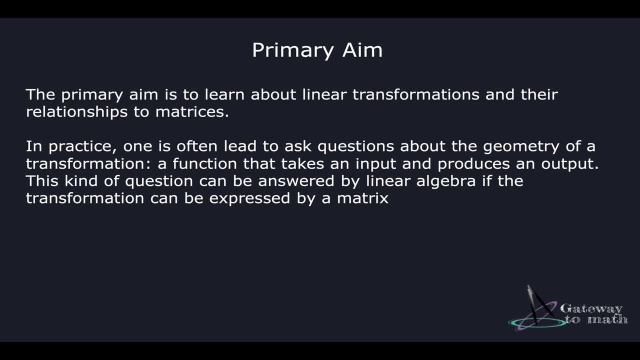 In practice, one is often lead to ask questions about the geometry of transformation, That is, a function that takes an input and produces an output. This kind of question can be answered by linear algebra if the transformation can be expressed by a matrix. So here what we are trying to do: the function, that is the f of x that we have. 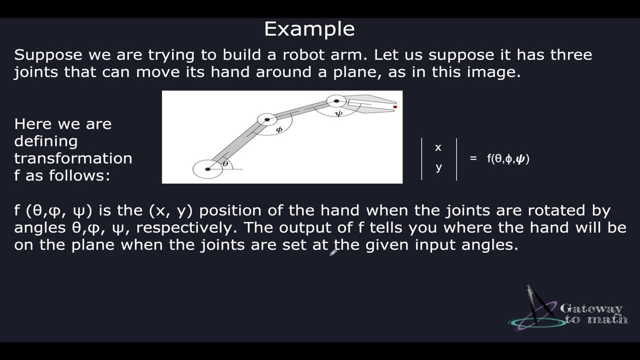 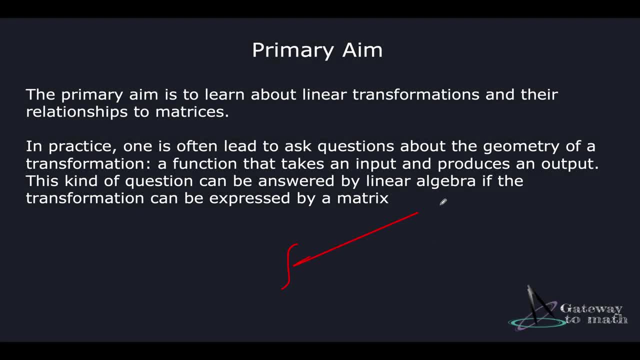 No, no, no, that's bad Here. So what we're trying to do here is the function which is f of Sorry, f of x. We're trying to replace this function as a matrix. So we are defining a function in the form of matrix and then using that matrix to multiply it with some form of vectors. 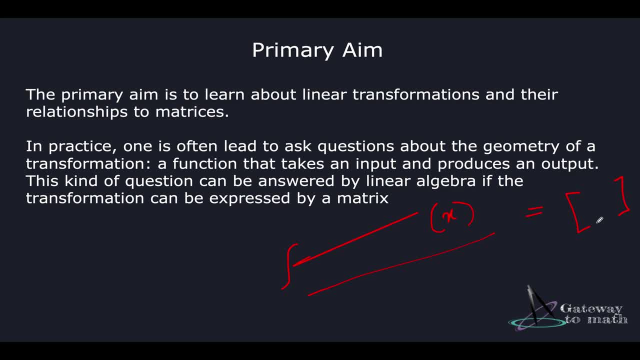 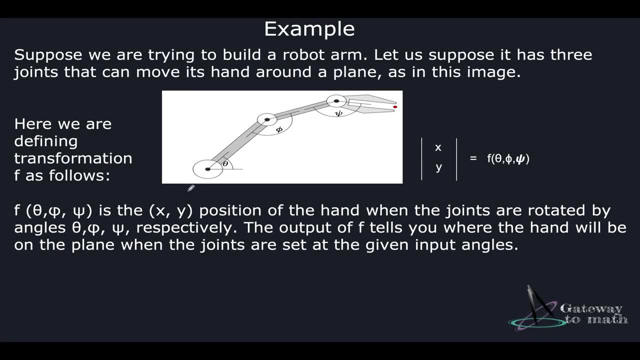 So we have some more space to see the output. This is what we're going to be doing throughout this session and the next few sessions. So let us take an example. here We have a robotic arm which is inclined over three angles on the three corners. 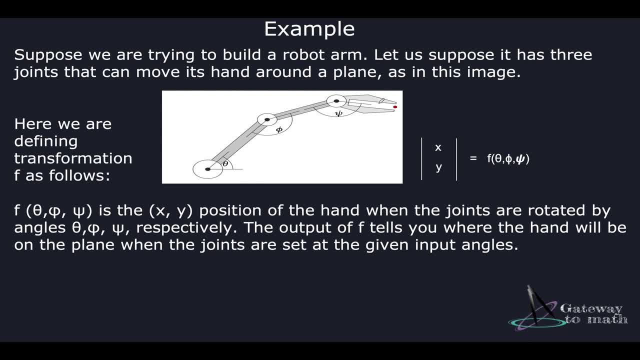 Depending upon what the value of these angles are, it defines the position of this robotic arm correct. So say, for instance, if my theta was more of an obtuse angle right, So then the position of this robotic arm would change. 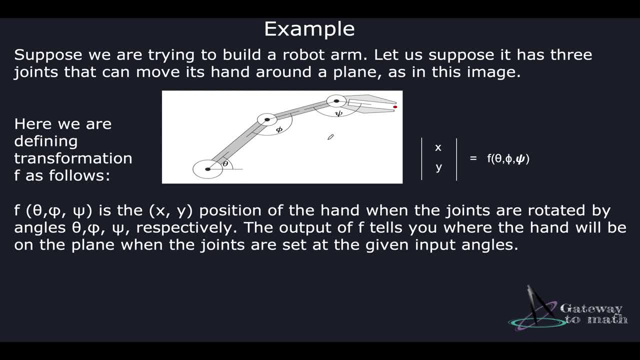 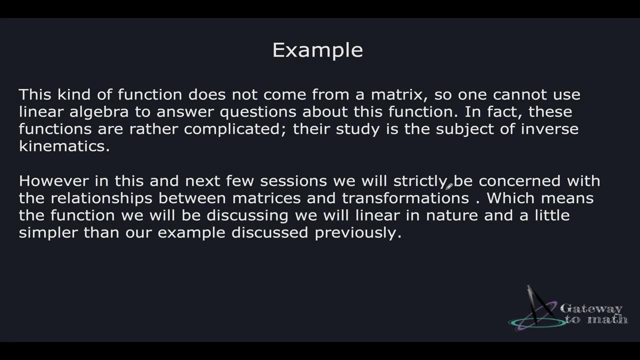 With respect x and y position, and so with the help of these three angles, at any point in time, i can predict where exactly the robotic arm will be right. so this is again an example of a function. so this example of a function is not linear in nature, it is rotational. this is not what we are. 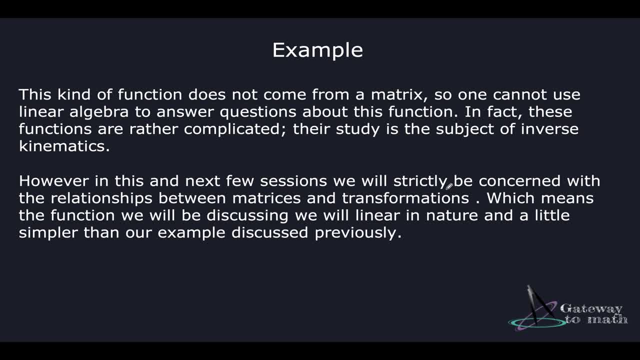 covering at this point in time. this comes under what is called as kinematics and inverse kinematics and we're not discussing it right now. i gave this example just to bring, just to let you guys know that we will be having a discussion about this topic a little later down the line. we will 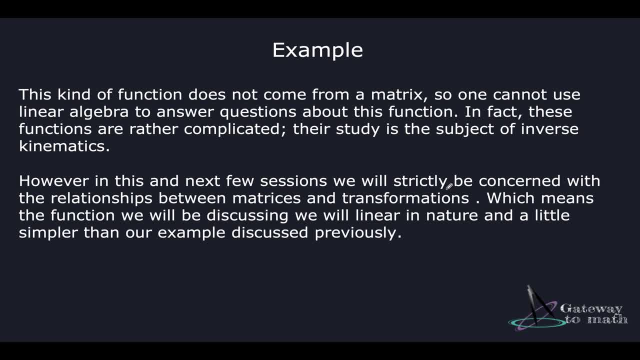 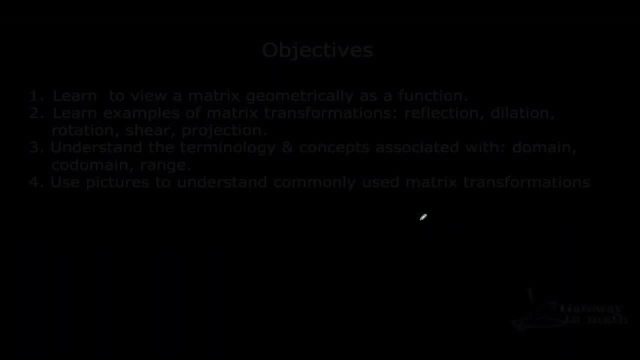 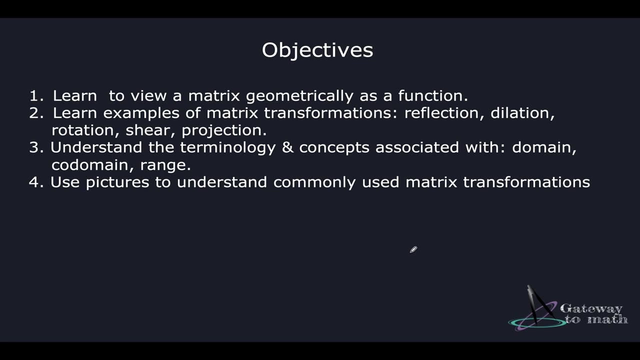 see how such a complex model can be applied to ai models and neural analysis. all right, that's why the example strictly for the next few slides, we will be focusing on functions which are linear in nature and we will be studying them briefly. so the objectives: learn to view a matrix geometrically as a function. learn examples of matrix transformation. 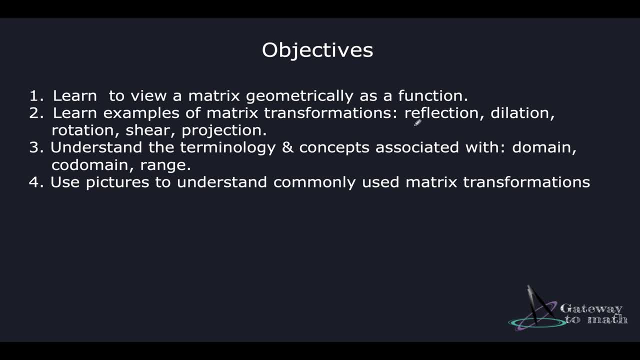 that is reflection dilation rotation shear projection. if you come from opencv background, you've done what is called as computer vision problems. you know what exactly a reflection dilation rotation shear projection stands for. just in case, if you do not have that background, that's fine too. you'll understand the underlining math behind these concepts. so when you decide to learn, 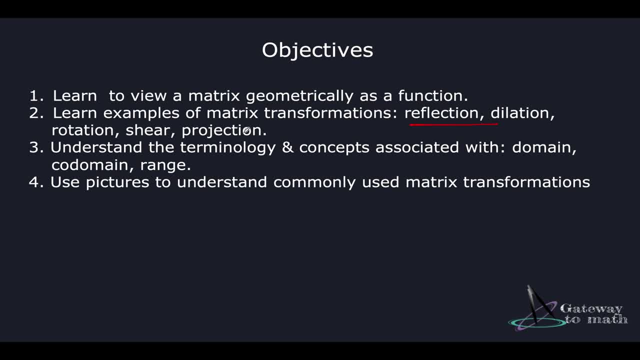 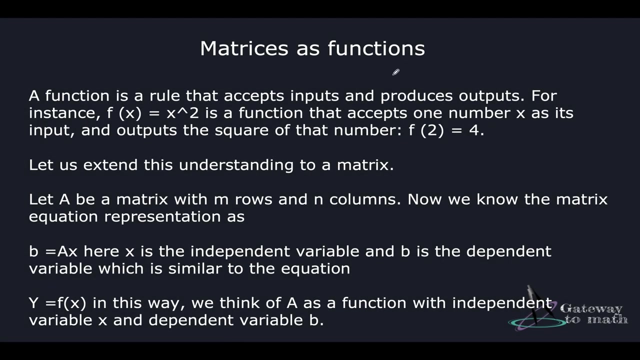 opencv or use computer vision programming stacks, you'll already know what these concepts are mathematically, understand the terminology and concepts associated with domain, co-domain and range. use pitches to understand commonly used matrix transformations. so these are some of the things we are going to be discussing in this session. now. matrices as a function. 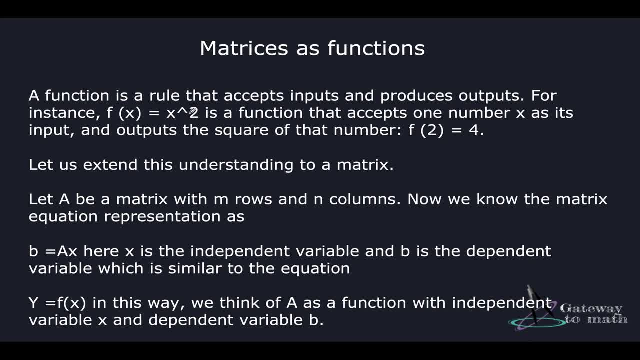 let us take an example here. i have a function f of x which is x squared. so if i put the value of fx x as, let's say, 2, then 2 squared is 4, so the output becomes 4. this is a function in itself. 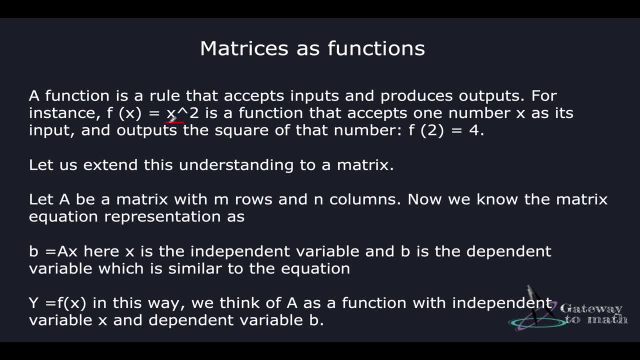 x here is an independent variable, because you can put any value here and then, depending upon the value you're putting here, you get the output, which is fx in this case. so this is a function. now let us map this representation to the matrix formation. all right, so we know from the matrix. 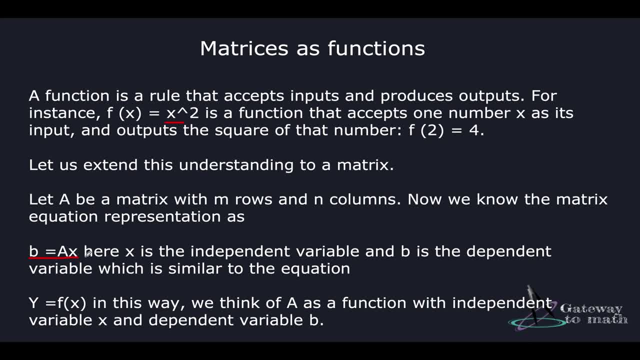 equation that p equals ax. we've seen this equation so many times since the start of the sessions and you already know how important this equation is here. a is the matrix, which has n number of rows and n number of columns. x is the independent variable and y becomes the dependent variable. 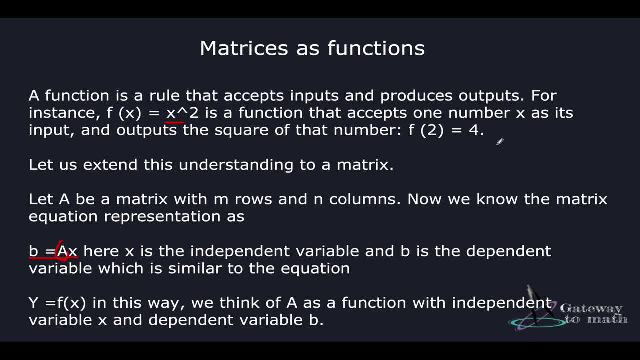 canonical form for this representation is actually: y equals fx, the same one, y equals fx. so here y is b, f of x is the function is matrix here, and x becomes the independent variable. so the representation of the functional aspect of this linear equation is represented by a matrix. 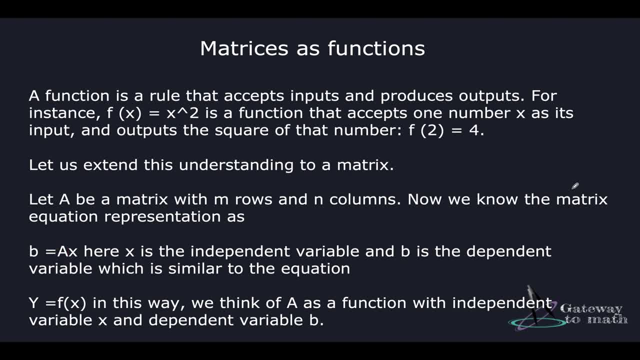 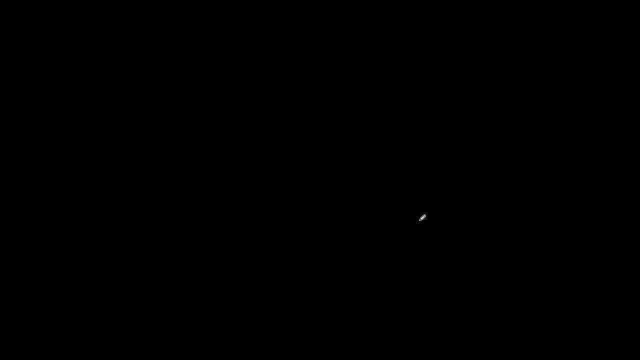 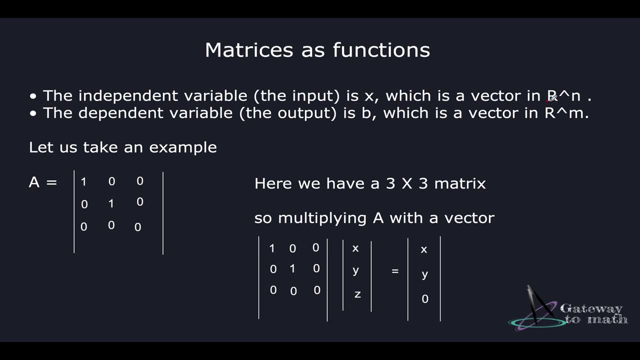 now, this is the relationship between the two. so let's see how it works. let's take an example. so the independent variable, that is the input, is a vector of r of n and the dependent variable, which is the output, is a vector of r of m. i don't have to repeat which was row and. 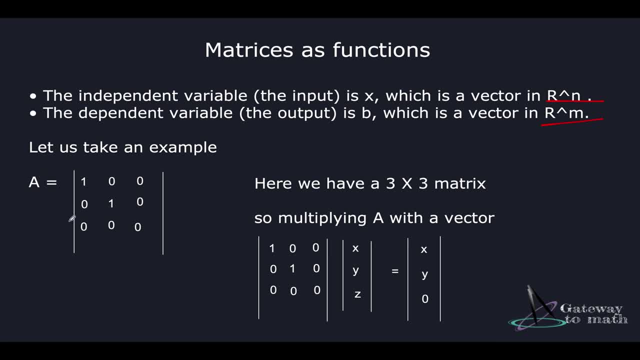 which was column, because i just said that. so this is a matrix here. this has three rows and three columns, so both n and m are three and three. since it's a, it's a matrix in three dimensional space, so the vector space coordinates will be x, y and z. 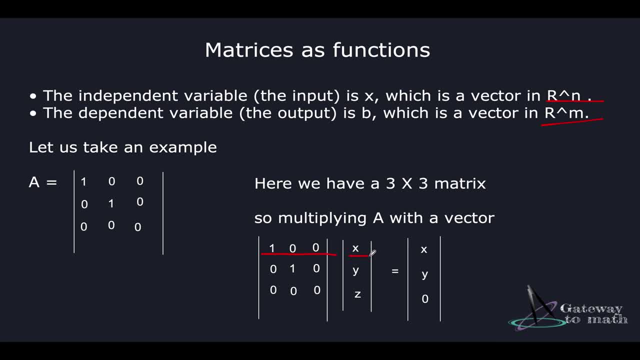 for the vector space coordinates will be x, y and z. so the vector space coordinates will be x, y and z. multiply the first row with x. just in case, if you've forgotten how the matrix multiplication works, i'll link the url to an older video which explains about the multiplication in the description box. 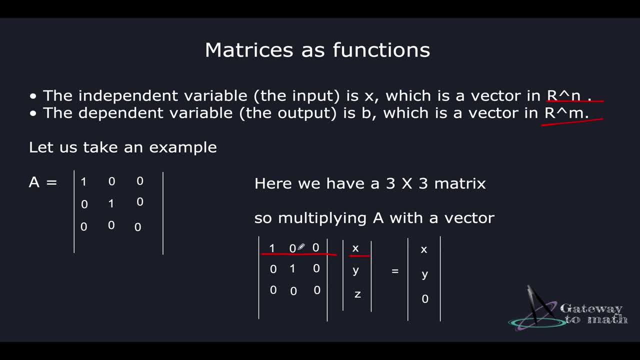 but again i'm doing a quick multiplication here: 1 multiplied by x plus 0 multiplied by y plus 0 multiplied by z is x. similarly, 0 multiplied by x plus 1 multiplied by y plus 0 multiplied by z is y, and then 0 multiplied by x is 0 plus 0 multiplied by y is 0, and then 0 multiplied by x is 0 plus 0, multiplied by y is 0. 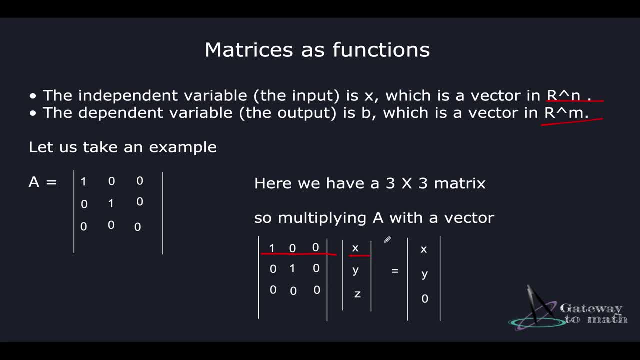 plus 0. So this is itself 0.. So we started with a vector which had three-dimensional space and then mapped it to a vector which is in just two dimensions. This is a very important problem. It might not be very intuitive at this point in time. what's so big about it that you've had? 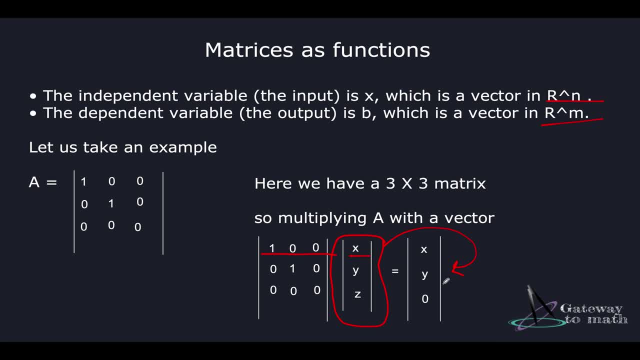 x, y, z as three. you know you had three vectors, three-dimensional vector, space, and then so what? you got them into two-dimensional space. What is the big deal? Right now, for me it's a little hard to explain. but when we apply this information- sorry, when we apply this understanding- to a real 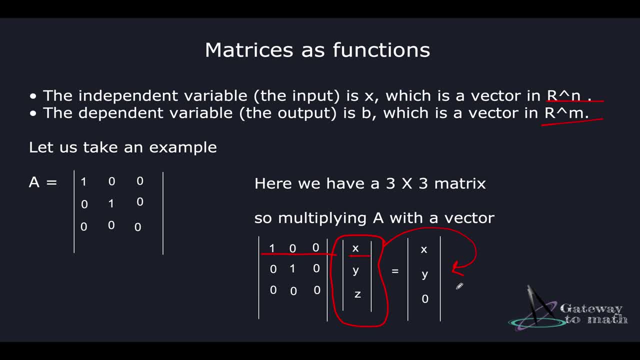 world problem. this will be quite clear why this is so important. because you know when you- I'm sorry I'm getting into the technicalities again, but just for the viewers who already have ML and AI background, we have dimensionality problem. right, We've heard things like dimensionality. 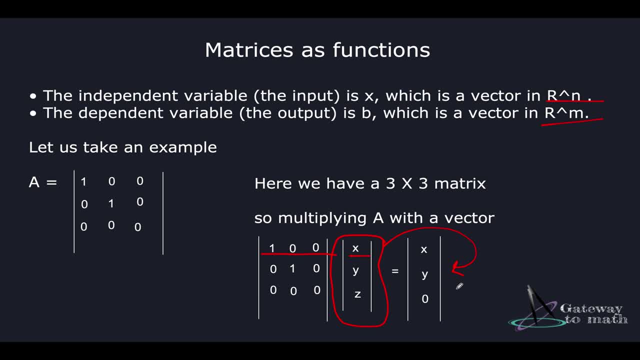 is a curse. and then you're supposed to break down the dimensionality to less number of dimensions because you have redundant column informations, correct? So that's what we try to do. but this reduction of dimension is very different than the dimensionality curse we talk about in ML. 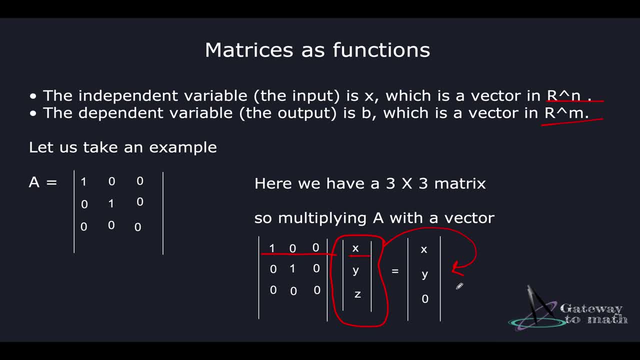 all right, That's because that's more of a parametric representation what I was talking in the previous sessions- that one column is actually dependent on other columns, so you can skip that column altogether. So this changing the dimensional space in itself is a very different problem statement. It's like 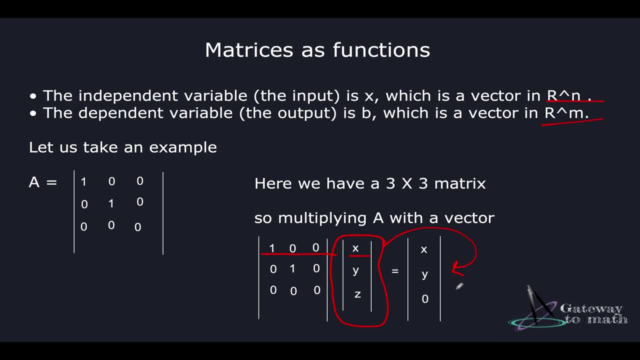 you have a 3D visual of something and then you are mapping it into 2D, So you have to map it in such a way that the information is still stored of the intricate information is still stored. So this has much more math involved and it's not similar to just reducing the number of columns. 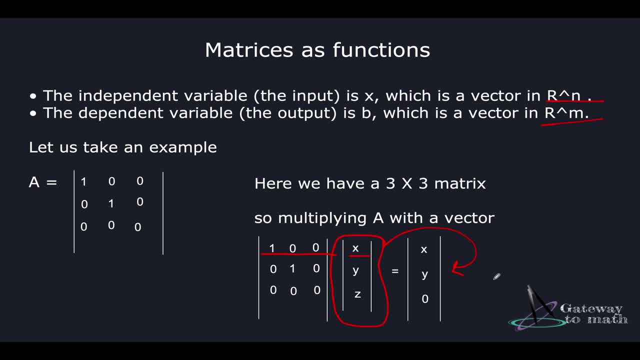 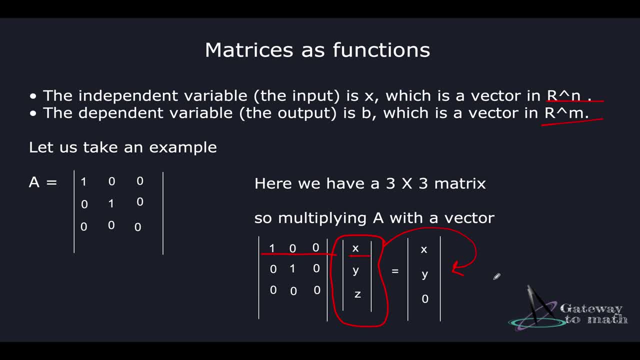 know how to do it. So they just don't know how to do it. So they just don't know how to do it. So now I just keep track where all the développer is place and also how many. OK guys, it is a. 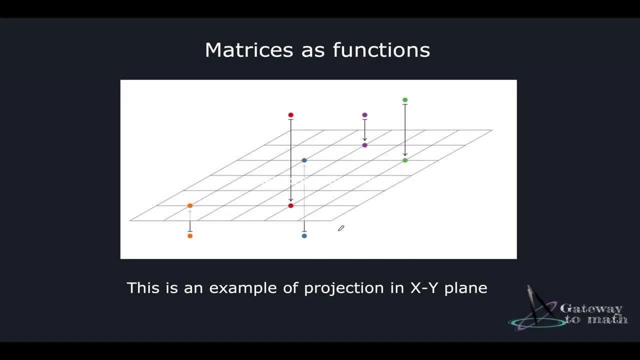 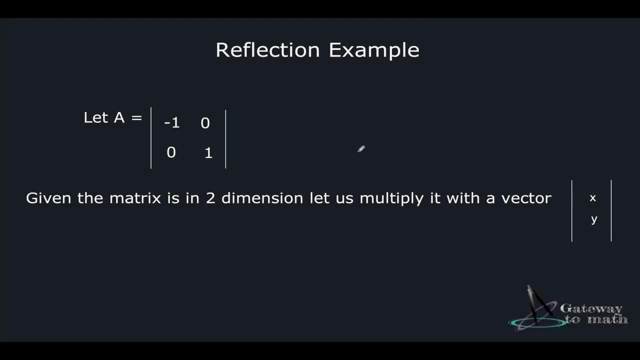 quick one. I just today briefly explain to you some of the actors way of pose거든 in a virtual set. So you see the body. not that different. the individual body is a sculpture. let's take an example which is reflection example. so now a equals minus 1, 0, 0, 1. this is a matrix. 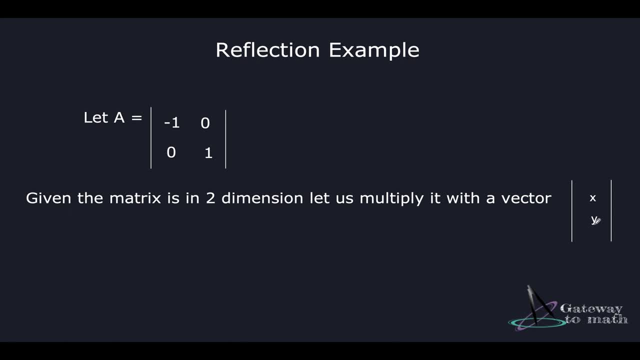 into dimension, so the vector space that we will be taking will also be a vector into a dimension which is x and y. let us multiply them. so minus 1, 0, 0, 1, you've multiplied it. minus 1 multiplied by x, plus 0 multiplied by y is 0. this becomes minus x, 0 multiplied by x plus 1 multiplied by y is y. 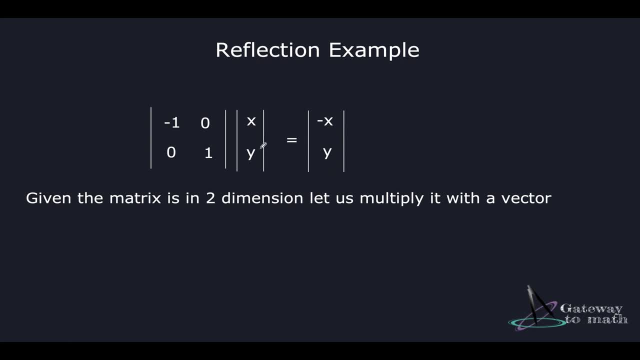 so this is your final output. this means that this has flipped on the x-axis. right, so it was. the image would have been first, or the value or the data set would have been on the positive side of x-axis, but after multiplying it with this function, it has it's on the negative side of. 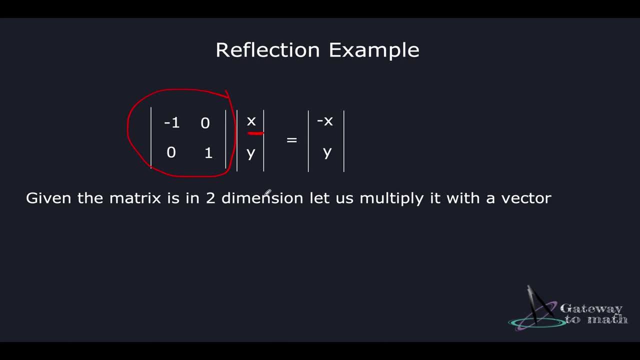 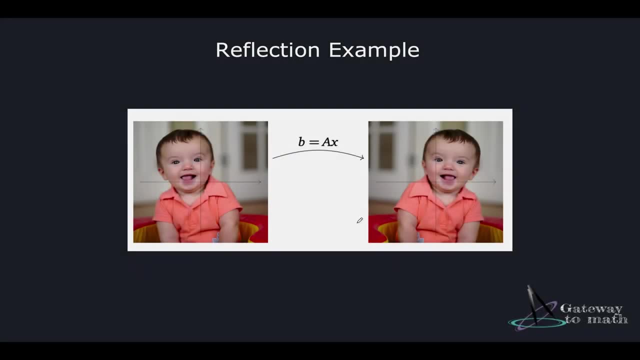 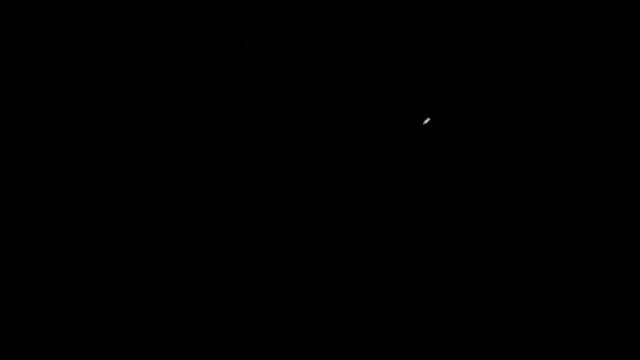 the x-axis. so it's there's a flip on the horizontal axis, on the x-axis. if we have to understand this with an image, this is how the image is right. so this is my x-axis here and this has actually been flipped on the x-axis, so this is called as reflection. now, what is important to see here is that such 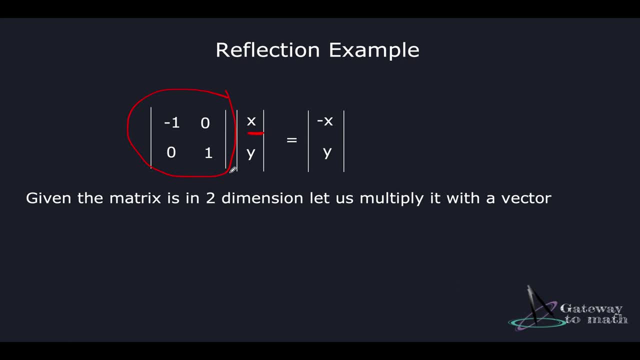 a conversion. if you're using any programming language, you just invoke a function in your code. you give the path of your image or you give the path of some data set that you have represented in the form of vector, space or anything of whatever you're holding your data set, it can be any data structure. you call that function and 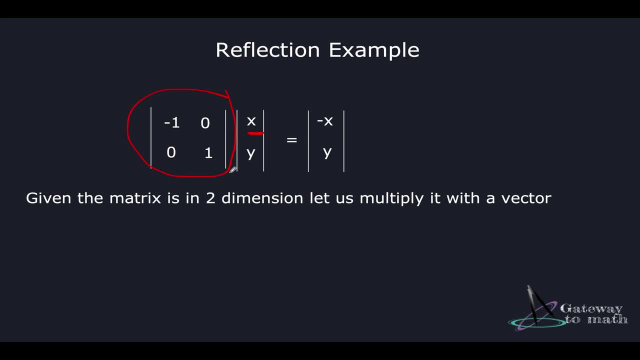 then you do a reflection of the values or the image inside that code, right? so underlining logic or the underlining maths of that function is actually a matrix whose values might be similar to something like this. so isn't it awesome that you're not just understanding that you're supposed 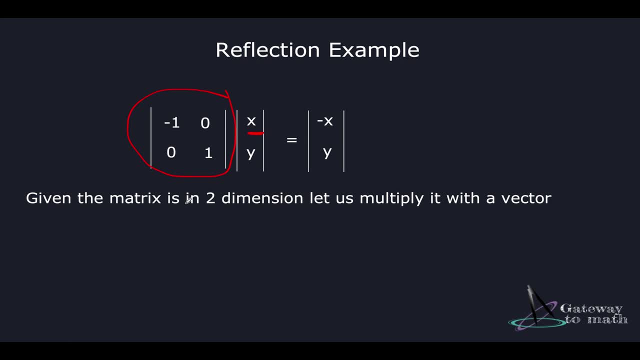 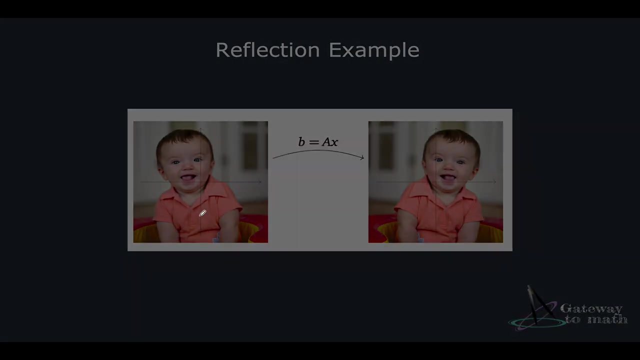 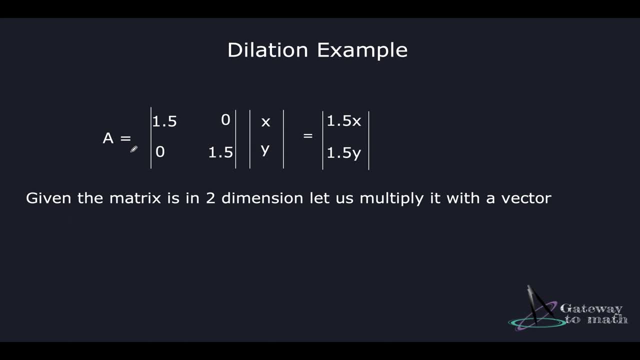 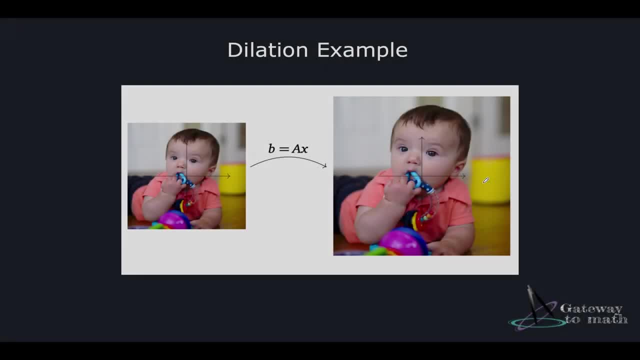 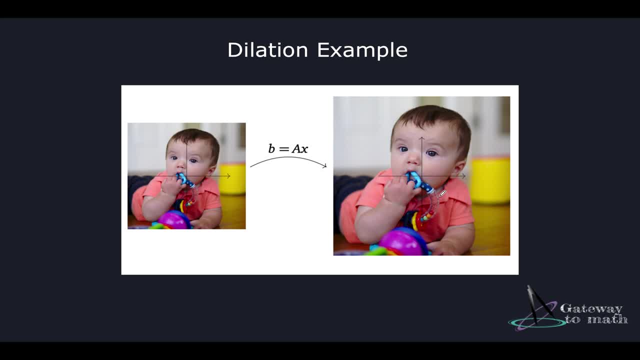 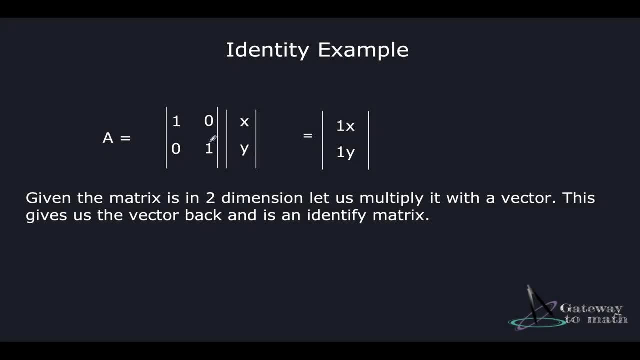 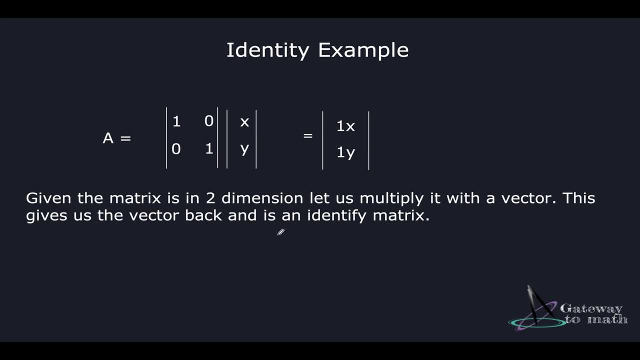 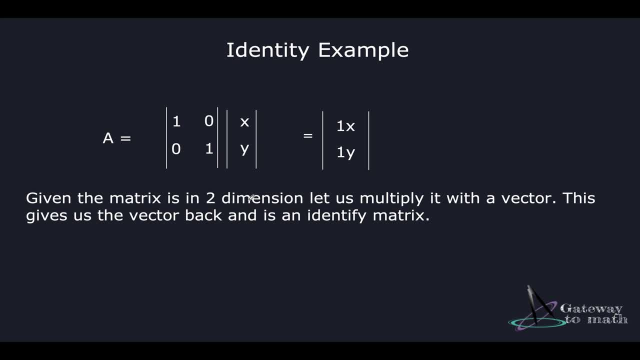 become more evident. but just to summarize an intuitive nature of an identity function, it's just like showing a mirror to person who's lost the path. all right, so you can just see yourself in the mirror. compare what you look in the mirror is what you want to be. if the answer equals, equals. 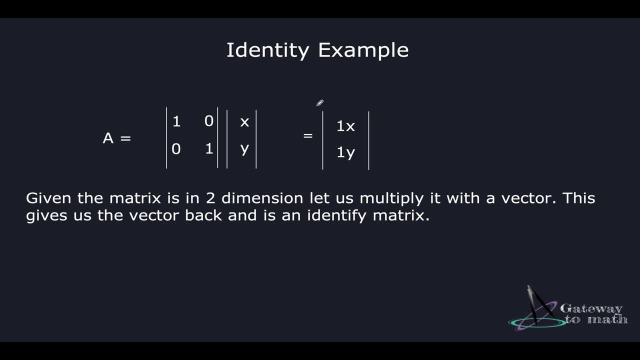 yes, keep doing what you're doing. the answer: equals equals no, then change it. similarly, in the case of machine learning, ai, whatever strategy has been implemented or whatever output you've got, you pass it through an identity function. if what you see is good enough and it can be fine-tuned and 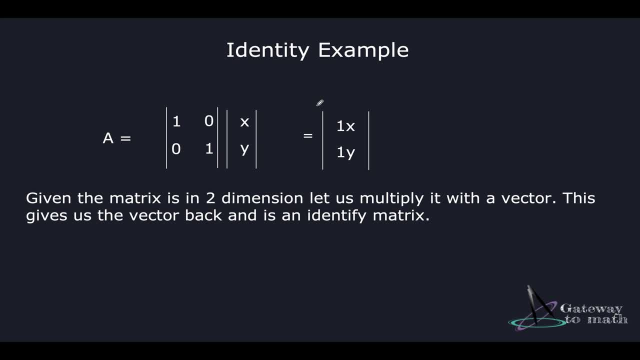 parametrized, then go ahead, follow the same strategy. but if it cannot be, then you are supposed to be changing your strategy. so that's where you're going to be using identity functions. still, if this is not clear, where exactly how the implementation aspects work with ml and ai. that's. 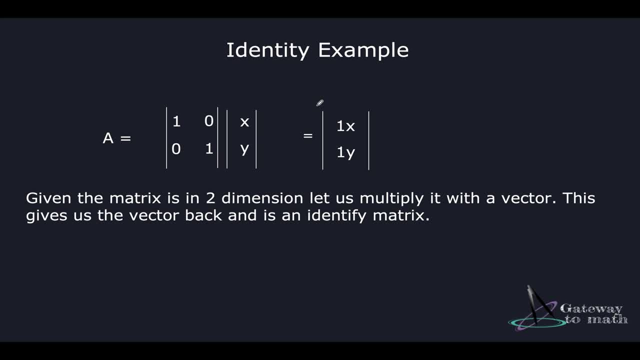 totally fine, because my aim is not to jump into ml and ai at this point. the aim is for you to get hold of the concept. so we're good. as long as you know what identity function or identity matrices do, we're good. the next example is rotation examples. the function for something like this will be 0 minus 1, 1 0 you. 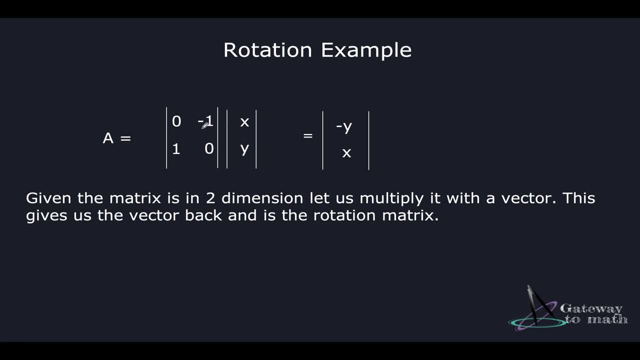 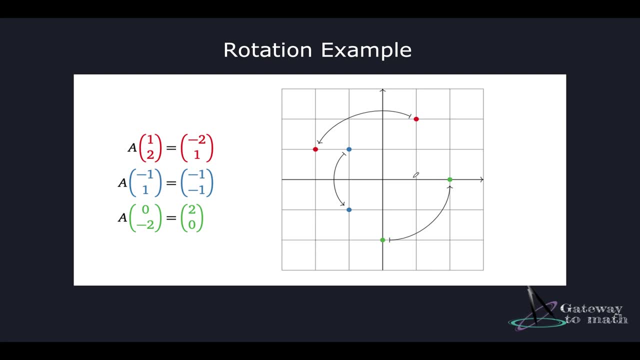 have x and y. so you multiply 0 with x is 0 plus minus 1. multiplied by y is minus y and this is x. so there's a rotation happening here. let's project this. so my input is 1 and 2, which is 1 on the x. 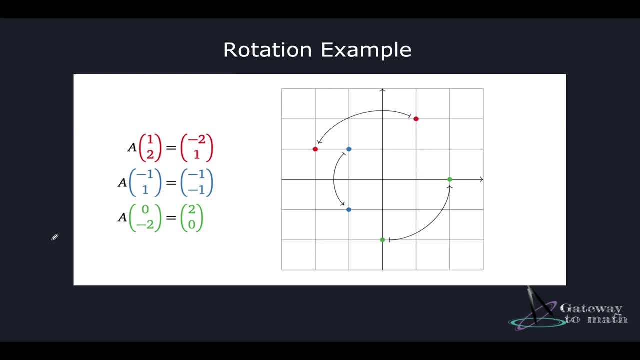 axis, 2 on the y axis, and then i rotated it so that means my y was on minus of x, so my minus y and x was my output. so this becomes minus 2 on the x axis and 1 on the y axis. this is a rotation by 90. 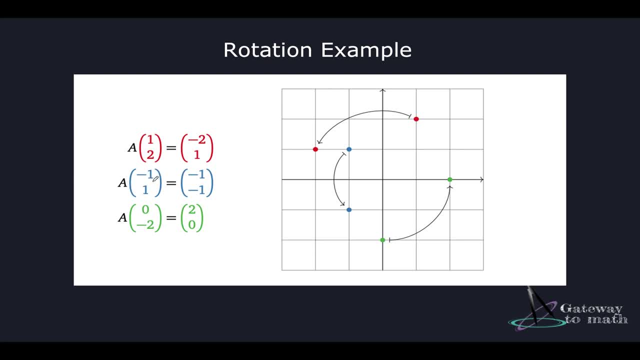 degree. similarly, this one, which is my input, is minus 1 on the x axis but positive 1 on the y axis. so minus 1 on the x axis and positive 1 on the y axis. my, my output is again swift. this comes on top with the minus sign and x is intact. so this becomes minus 1 here and this becomes minus 1 here. 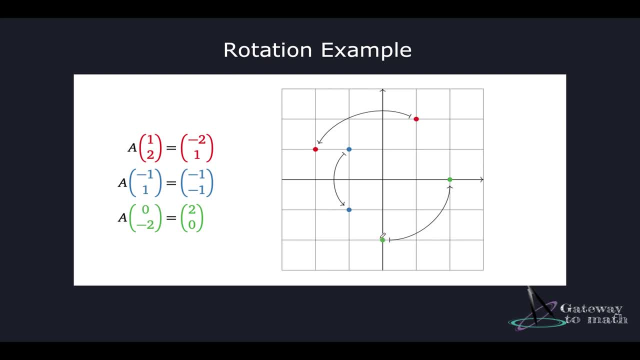 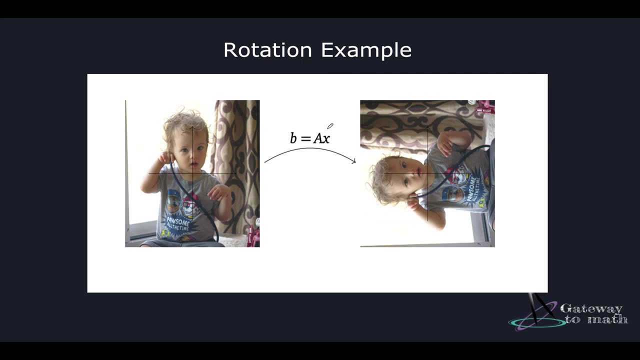 and in this example, when a is 0 minus 2, which is somewhere here, and then when you're projecting it again, it is rotated and the values come on the x axis. so this is a rotation example of a 90 degree rotation. that was an example of a 90 degree rotation. so here you see an image in this format and it has been rotated by. 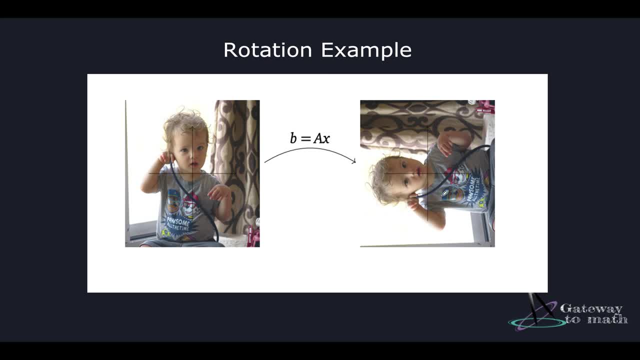 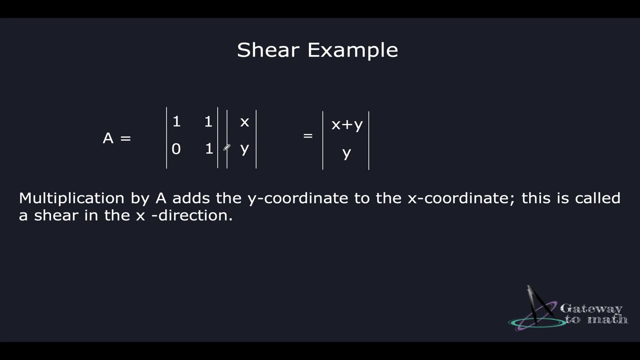 90 degrees, pretty much. so now you know, if you guys are mac users, how underlining mac mac os is actually making a conversion. isn't that really awesome? not that much. what's the big deal? yes, yeah, i think so too. no big deal. a equals one, one, zero, one x and y, so you multiply. it's extended. on the: